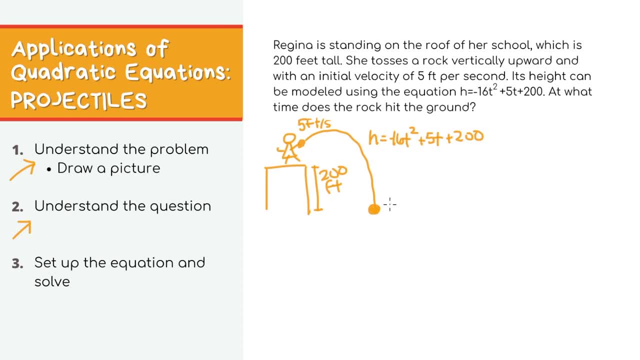 Well, logically, the rock hits the ground when the height is equal to 0, because the rock will be 0 feet off the ground. Now for step 3, when we set up our equation, we can plug in H equals 0 and solve for T to get the time when the height equals 0. 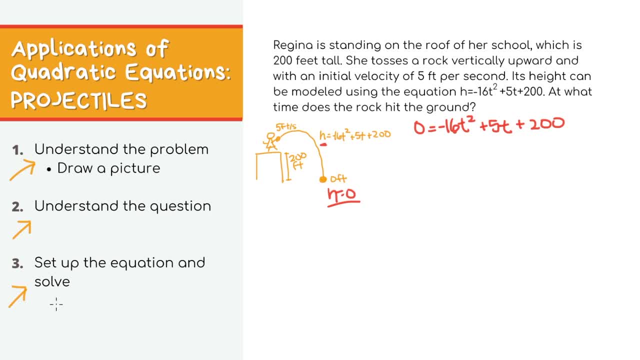 When it comes to quadratic equations, there are a couple ways to solve it. If you're not familiar, I have another video on four ways to solve quadratic equations, but I usually go either for factoring or the quadratic formula. And just looking at this equation, there's no way I'll be able to factor this. 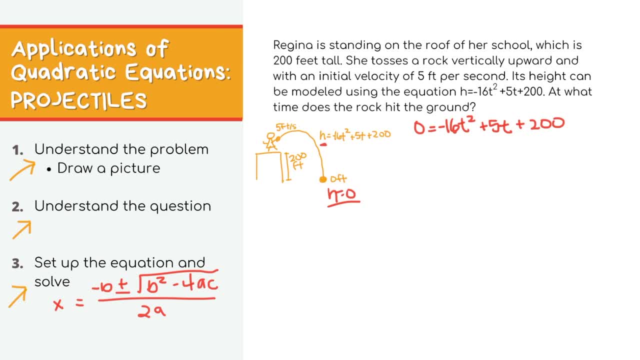 so I'll use the quadratic formula, which I've copied down here, To solve. we'll find our A, B and C values, then plug it into the formula And, just like magic, we have our answers. Notice, we'll end up with two. 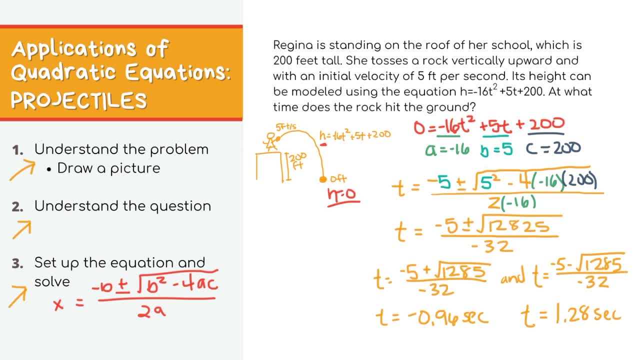 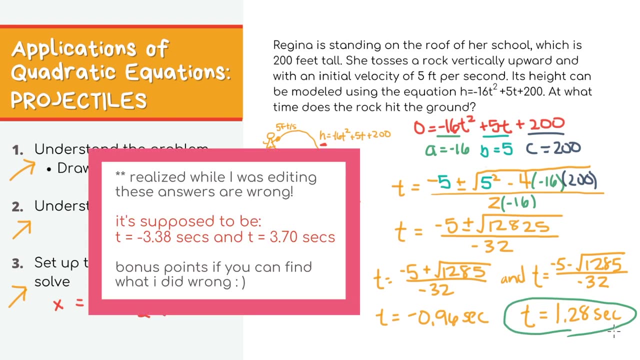 answers because of the plus or minus in the quadratic formula, but only one will make sense logically. This one is negative, which doesn't make sense unless you can travel back in time. So this is our final answer. Up next we have these problems where people are building fences to enclose their gardens or animals. 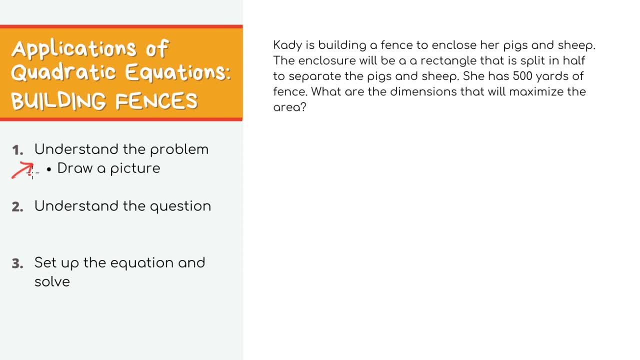 Let's first understand the problem. In our case, we have our girl, Katie, who has some pigs and sheep. she needs to build a fence, for It's going to look like a rectangle with fence running down the middle to separate the animals, And she has a total of 500 yards of fence. 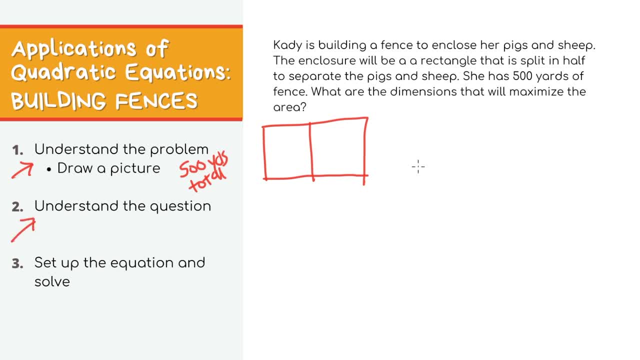 The question is what dimension will maximize the area, Or in other words, what is the length of each side of the fence that will give you the biggest space inside the fence. Depending on how you build your fence, you might get bigger or smaller areas. 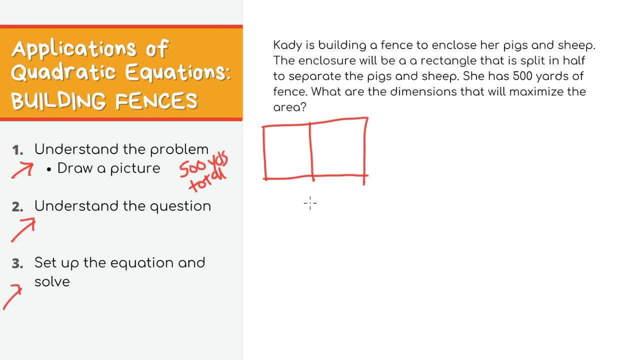 Let's now set up the equation. We're trying to figure out the area which, if you remember, is just length times width, So we'll use this equation as a starting point. We don't know the length or width yet, so I'll label the width as x. 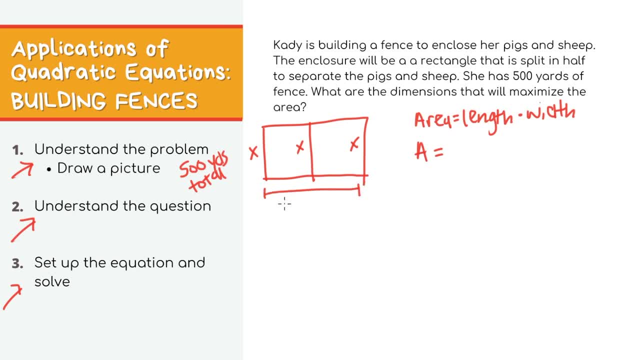 Then we need to write the length in terms of x, because we can't have three variables in an equation. We won't be able to solve it. We need to write the length in terms of x, because we can't have three variables in an equation. We won't be able to solve it. 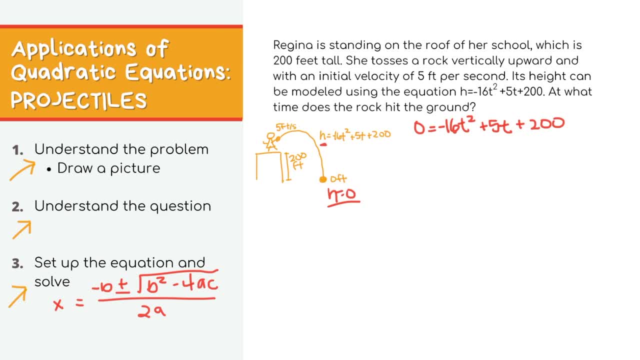 so I'll use the quadratic formula, which I've copied down here, To solve. we'll find our A, B and C values, then plug it into the formula And, just like magic, we have our answers. Notice, we'll end up with two. 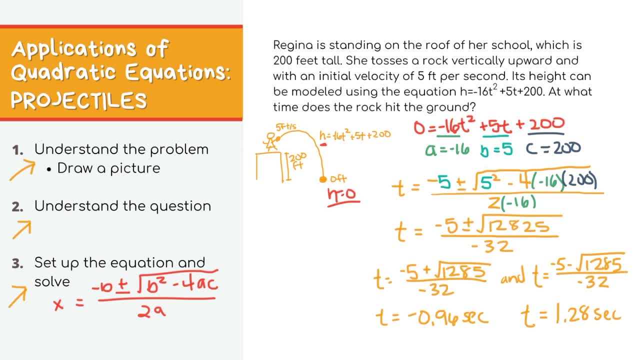 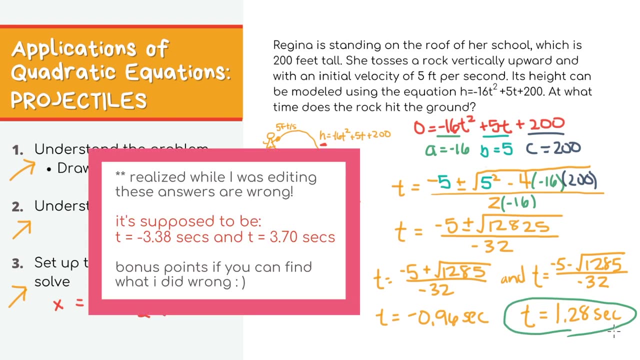 answers because of the plus or minus in the quadratic formula, but only one will make sense logically. This one is negative, which doesn't make sense unless you can travel back in time. so this is our final answer. Up next we have these problems where people are building fences to enclose their gardens or animals. 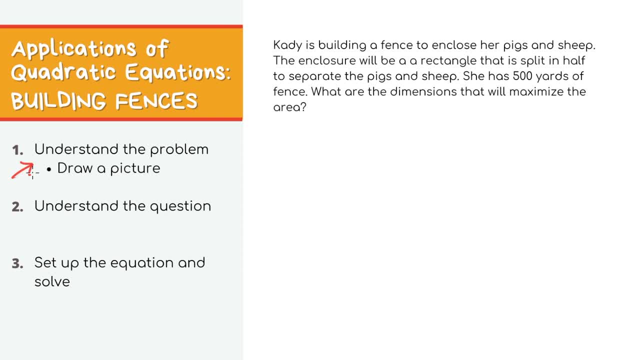 Let's first understand the problem. In our case, we have our girl, Katie, who has some pigs and sheep. she needs to build a fence, for It's going to look like a rectangle with fence running down the middle to separate the animals. 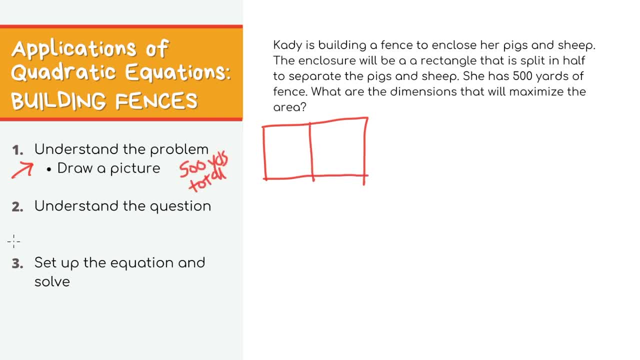 And she has a total of 500 yards of fence. The question is what dimension will maximize the area, Or in other words, what is the length of each side of the fence that will give you the biggest space inside the fence? Depending on how you build your fence, you might get bigger. 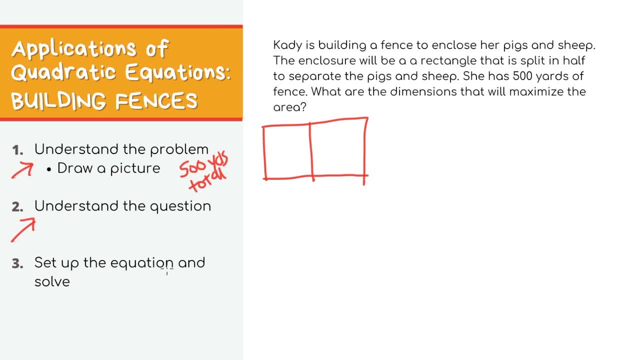 or smaller areas. Let's now set up the equation. We're trying to figure out the area which, if you remember, is just length times width, So we'll use this equation as a starting point. We don't know the length or width yet, so I'll label the width as X. 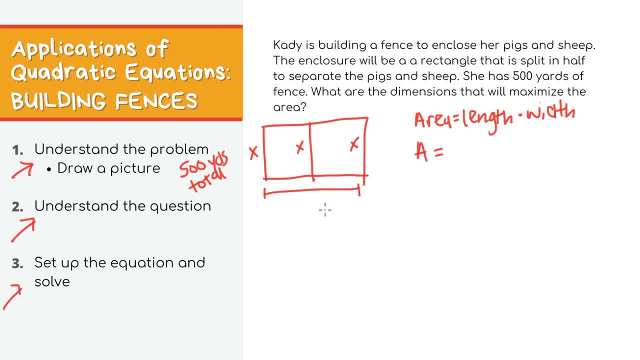 Then we need to write the length in terms of X, because we can't have three variables in an equation, we won't be able to solve it. solve it So to write it in terms of x. you can think of it like we had a total of 500. 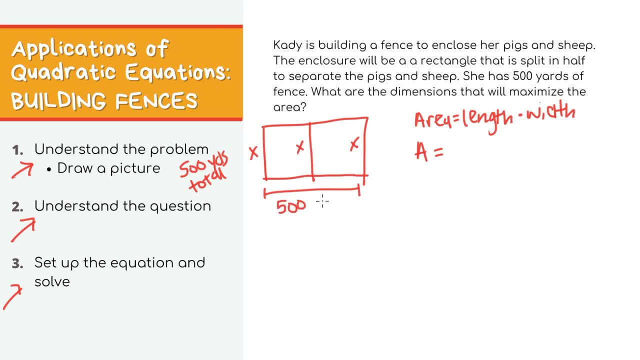 yards to start with, but we've already used up three of these for the width, So we can subtract three x's And because we have two of these long sides, we have to divide it by two and the other long side will have the same length If you plug everything in. 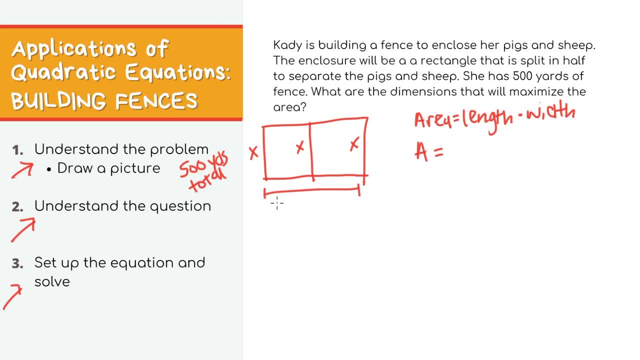 We need to write the length in terms of x, because we can't have three variables in an equation. We won't be able to solve it, So to write it in terms of x. you can think of it like we had a total of 500 yards to start with. 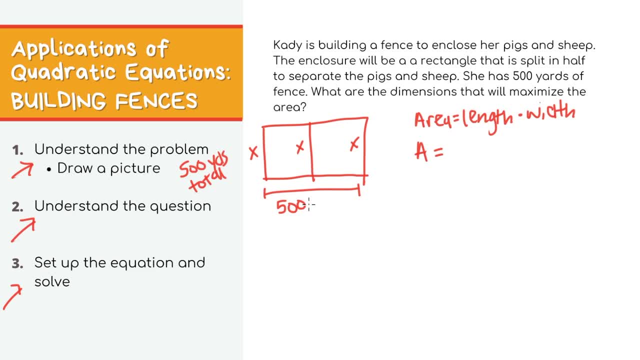 but we've already used up three of these for the width. So we can subtract three x's And because we have two of these long sides, we have to divide it by two And the other long side will have the same length. If you plug everything in now, we have the area as a function of x. 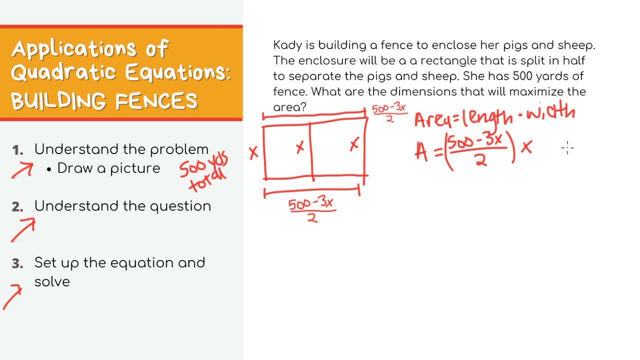 and if we clean up the equation and distribute, we'll get the area equals negative three over two x squared plus 250 x. When we're solving, it's asking: how do we maximize the area? Well, if you remember what a parabola looks like, 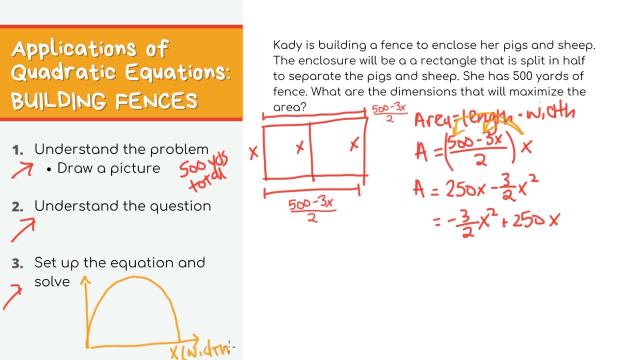 the x-axis will represent our width and the y-axis represents our area. So you can tell that here is where the area is the biggest, because the parabola is the tallest at this point. the vertex which we happen to know, the formula of: 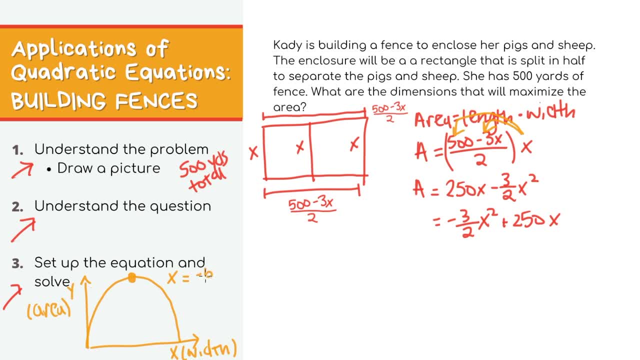 where the x-value of the vertex is found at negative b over 2a. When we plug in our a and b values from the equation, we'll get the x-value 83.3 yards. To get the length, let's plug it back into this expression. 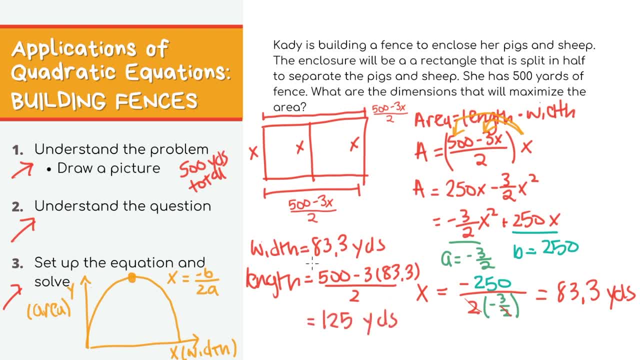 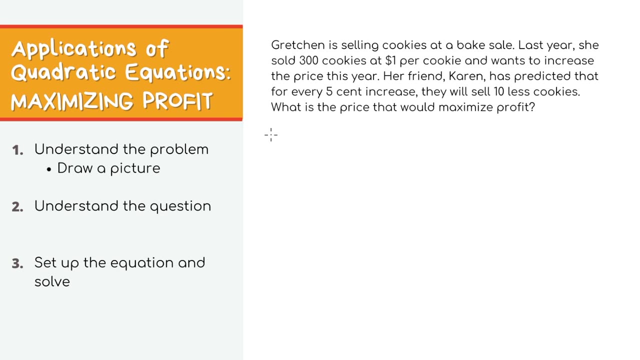 83.3 for x, we get 125 yards as our length. Those are our final dimensions where we'll get the maximum area. Our last type of questions is about maximizing profits. Usually people are selling gym memberships or car washes or whatever. 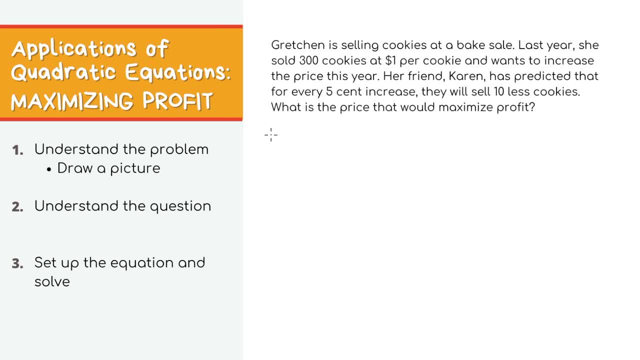 and they're trying to price it so that they get the most profit, which I mean. who doesn't want to maximize profit? So let's take a look at this example. Let's say you're selling cookies at a bake sale. She was pretty good last year because she sold 300 cookies for $1 each. 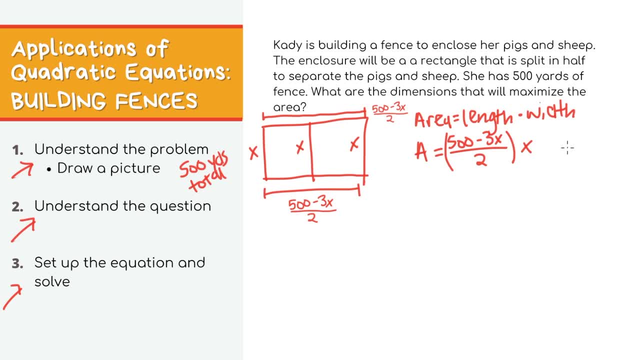 now we have the area as a function of x And if we clean up the equation and distribute, we'll get the area equals negative three over two x squared plus 250 x. When we're solving, it's asking: how do we maximize the area? Well, if you remember what, 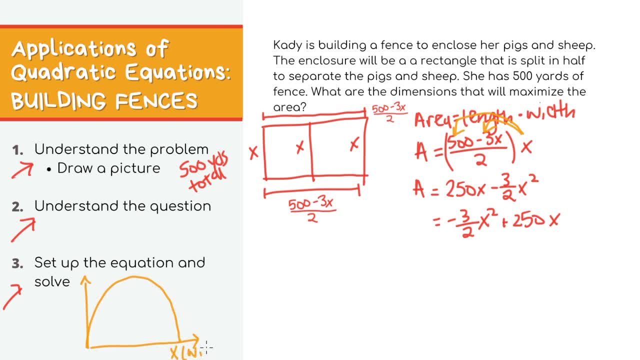 a parabola looks like the x-axis will represent our width and the y-axis represents our area. So you can tell that here is where the area is the biggest, because the parabola is the tallest at this point. the vertex which we happen to know, the formula of where the x 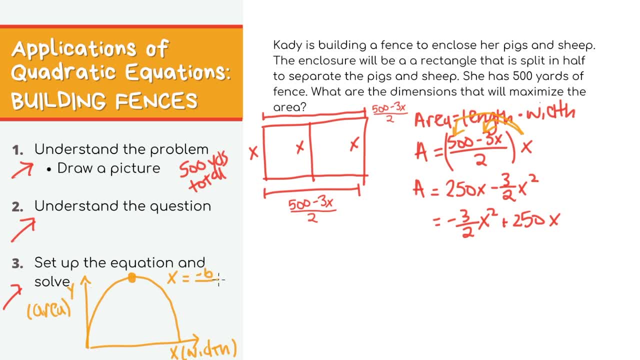 value of the vertex is found at negative b over 2a. When we plug in our a and b values from the equation, we'll get the x value: 83.3 yards. To get the length, let's plug it back into this expression. 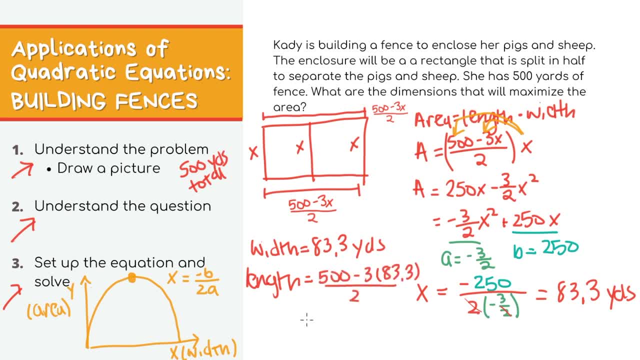 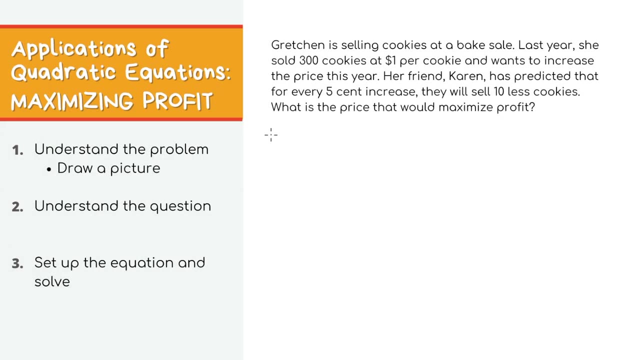 So plugging in 83.3 for x, we get 125 yards as our length. Those are our final dimensions, where we'll get the maximum area. Our last type of questions is about maximizing profits. Usually people are selling gym memberships or car washes or whatever and they're trying to price it so that they get the most profit. 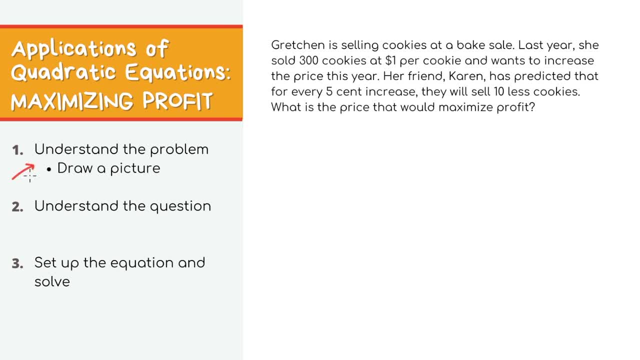 which I mean who doesn't want to maximize profit. Here we have Gretchen, who's selling cookies at a bake sale. She was pretty good last year because she sold 300 cookies for $1 each, but she's getting a little greedier this year. 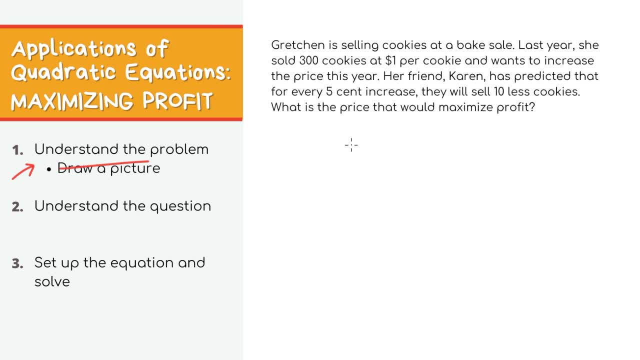 and she wants to charge more. Apparently, her friend Karen ran the numbers and somehow determined that for every 5 cent increase she would sell 10 less cookies. Now the question is: what price should she sell her cookies to make the most money? Obviously you can't. 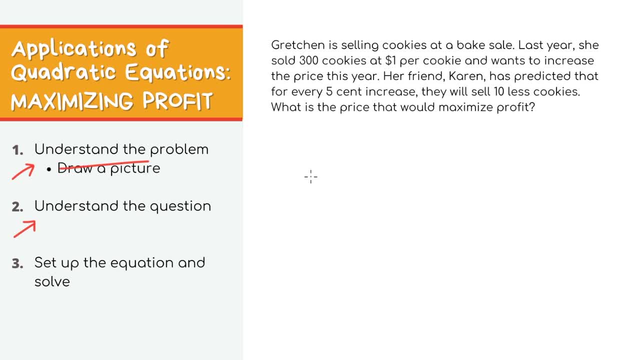 price it too high, because no one will buy $10 cookies, but if you price it too low, you'll just make the same amount of money you made last year. When we're setting up the equation, just remember that revenue, also known as the amount of money you make. 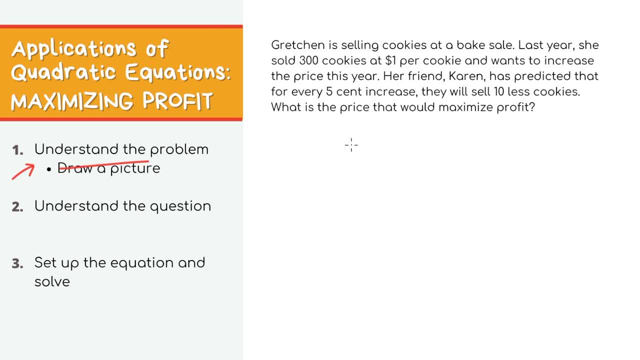 but she's getting a little greedier this year and she wants to charge more. Apparently, her friend Karen ran the numbers and somehow determined that for every 5 cent increase she would sell 10 less cookies. Now the question is: what price should she sell her cookies to make the most money? 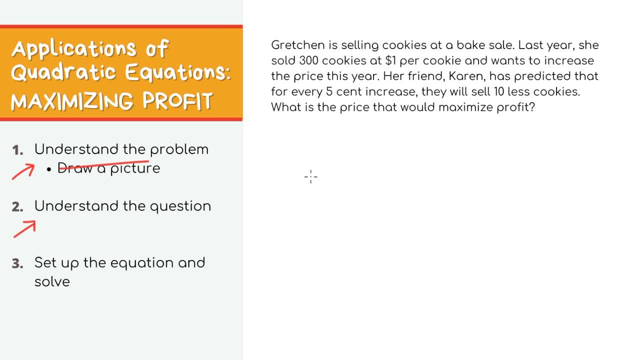 If you're selling cookies for $1,, no one will buy $10 cookies, but if you price it too low, you'll just make the same amount of money you made last year. When we're setting up the equation, just remember that revenue. 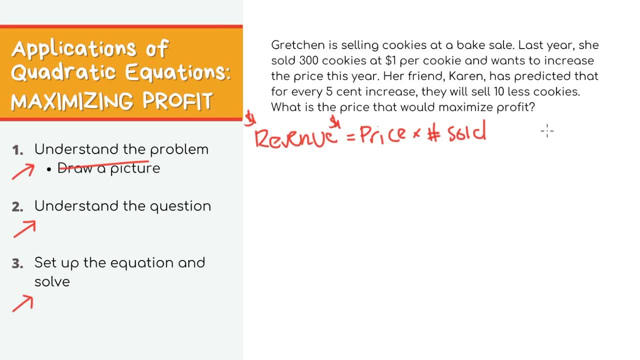 also known as: the amount of money you make equals the price times the number of cookies sold. For example, if you sell 5 cookies for $1, the amount of money you make, or the revenue, is 1 times 5,, which is $5.. 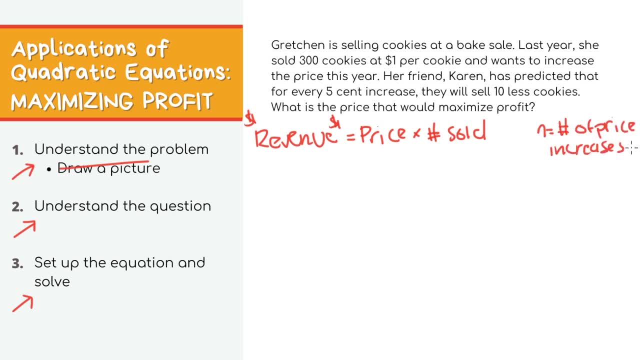 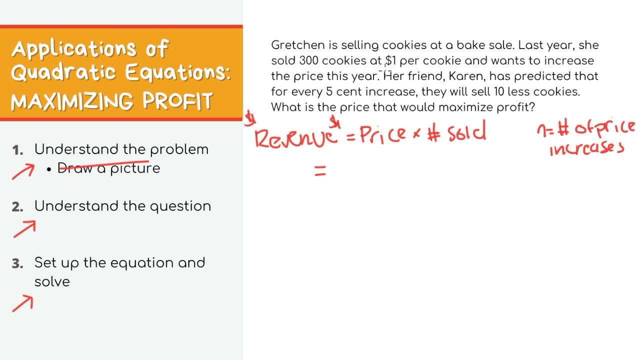 so the new price is $1.10.. So, going back to the formula, the price will be $1,, which is your starting point, and you're thinking about increasing the price by 5 cents times n amount of times Then for the number of cookies. 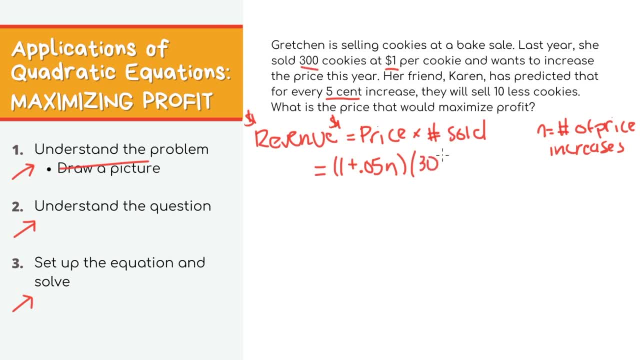 you have your starting point 300,, but you'll lose 10 cookies for each time you increase the price. This is our equation, which I'm just going to distribute and put it in standard form. Now this is another maximizing question. 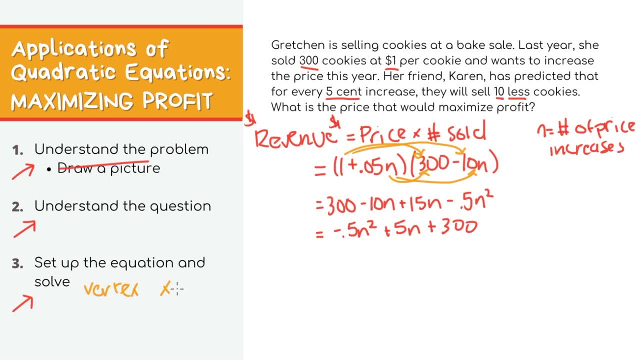 so we need to find the vertex of this equation. like we did in the last example, Let's plug in our a and b values into the vertex formula. Simplifying, we'll get n equals 5, which means that we should increase the price by 5 increments. 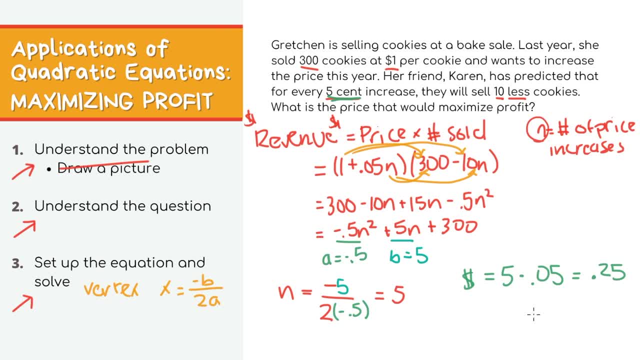 5 times 5 cents, which equals 25 cents. So it's basically saying that we should increase our price by 25 cents, which leaves us with a total of $1.25 per cookie, which is our final price to maximize profit. 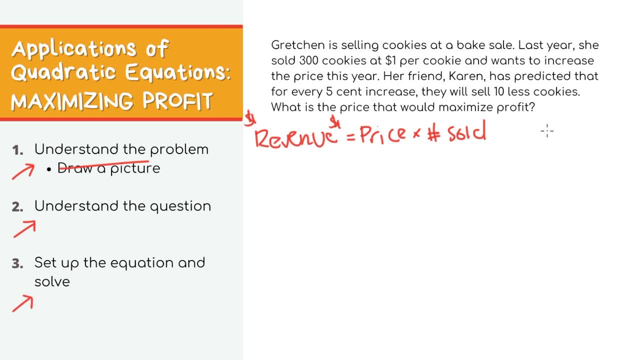 equals the price times the number of cookies sold. For example, if you sell five cookies for $1, the amount of money you make, or the revenue, is 1 times 5,, which is $5.. We'll write the formula in terms of n, where n is the number of times you increase the price For. 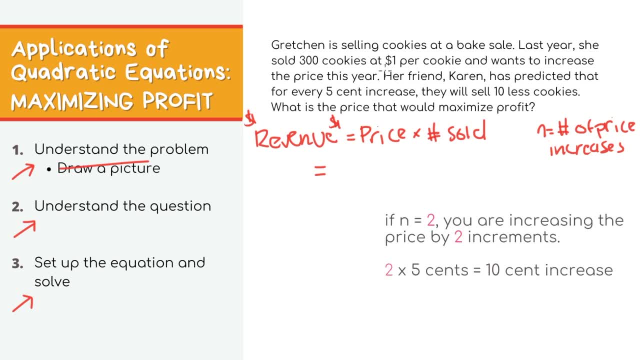 example, if n equals 2,, you're increasing the price by two increments, so the new price is $1.10.. So, going back to the formula, the price will be $1, which is your starting point, and you're thinking about increasing the price by 5 cents times n. amount of times. 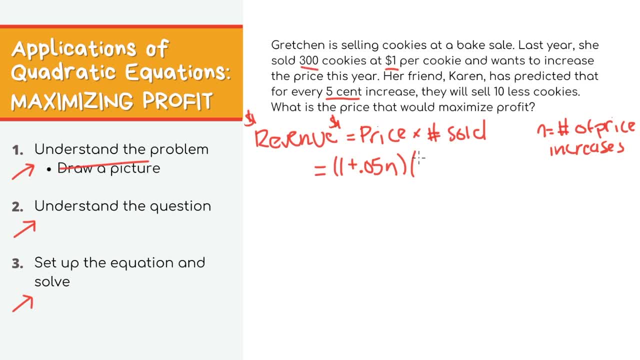 Then, for the number of cookies, you have your starting point- 300, but you'll lose 10 cookies for each time you increase the price. This is our equation, which I'm just going to distribute and put it in standard form. Now, this is another maximizing question, so we need to. 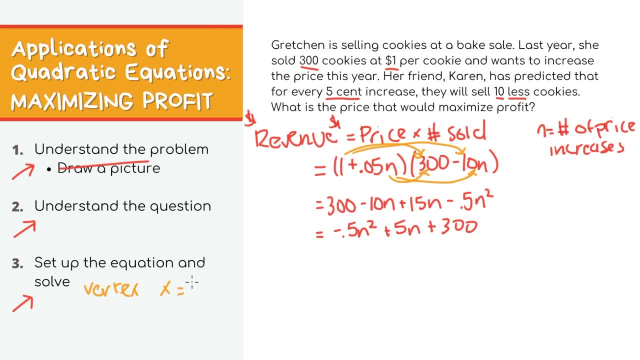 find the vertex of this equation. like we did in the last example, Let's plug in our a and b values. Let's plug in our a and b values into the vertex formula. Simplifying, we'll get n equals 5, which means that we should increase the price by 5 increments, 5 times 5 cents, which. 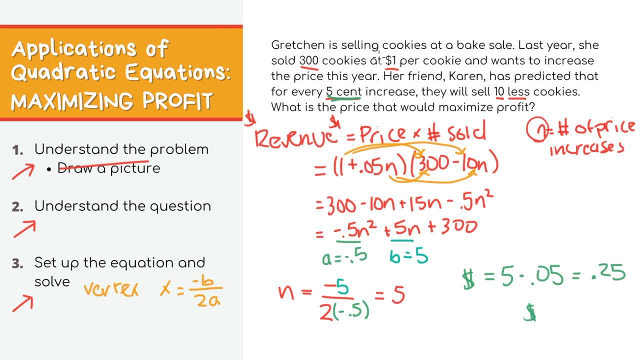 equals 25 cents. So it's basically saying that we should increase our price by 25 cents, which leaves us with a total of $1.25 per cookie, which is our final price to maximize profit. All right, that's it. Thanks for watching this video on applications of quadratic equations. 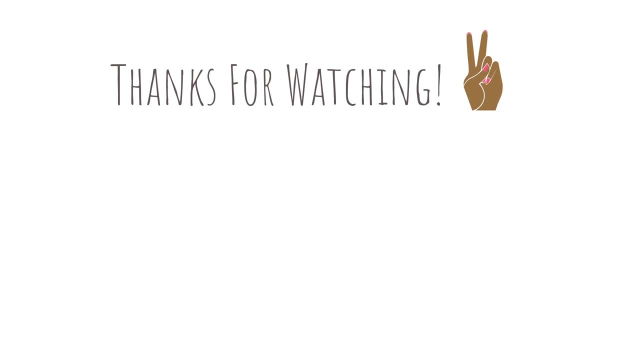 If this was helpful, be sure to give this video a thumbs up and subscribe for more math videos. See you in the next one.